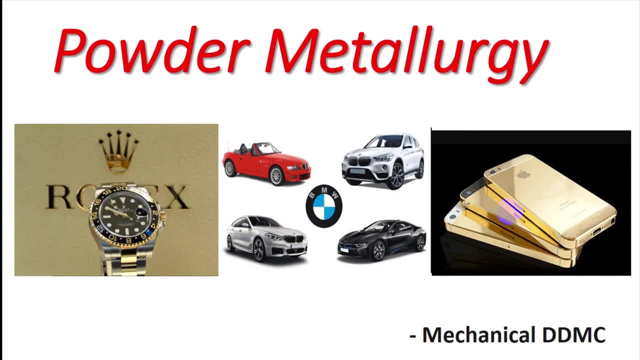 learn much from this video. Before starting this video, I want to explain something about you: Why some companies or some products are too expensive compared with other. Take an example of the Rolex brand, Rolex watch. Why it's too expensive compared with other watches. Too much expensive compared to other cars, And why iPhones are too much expensive compared with other mobiles which are providing similar features. The only answer is the quality that these brands are providing. It means people are not just seeking the features. they are seeking quality from the products. That's why they're spending too much money in these. 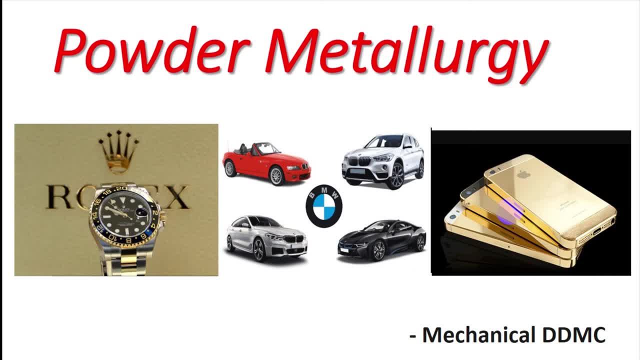 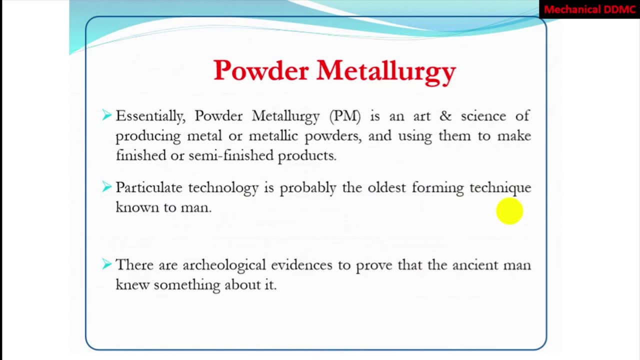 brands is much important. now start this video. turn our concept to powder metallurgy. the powder metallurgy. what is powder metallurgy? essentially, powder metallurgy is an art and science of the producing metal or metallic powders and using them to make finish or semi-fence for means. powder metallurgy concept itself gives that it is related to the powder. 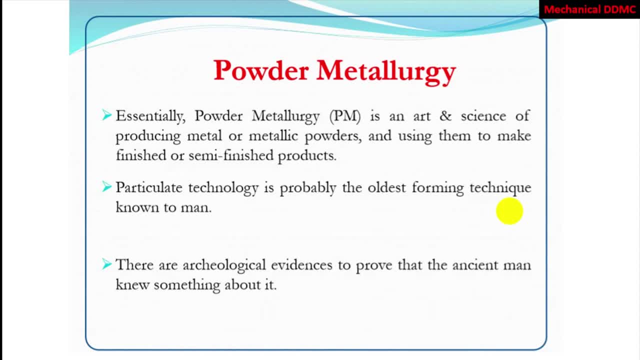 and metallurgy means something metal and dispersion means in powder metallurgy we are using the powder of the metals is a raw product for our processing, okay, and we are mixing them and producing some parts, and in further video i will explain this process step by step again. 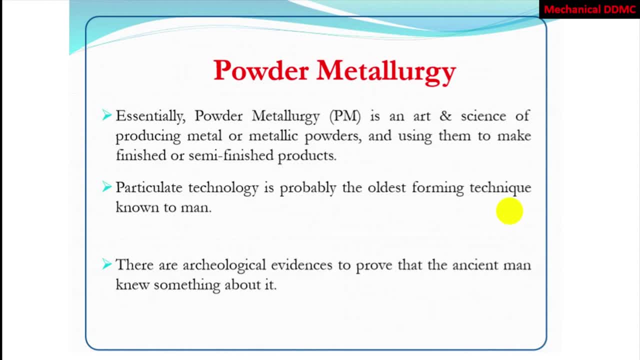 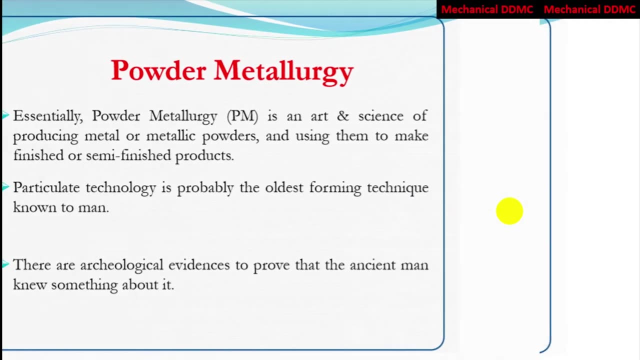 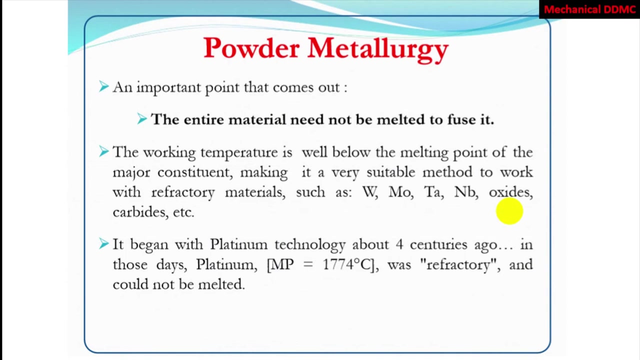 the powder metallurgy is a new concept in this scenario, but the terms used in powder metallurgy and the thinking comes from previous. it means from ancient man knew something about it. powder metallurgy is an important point that comes out. the entire metal need not to be melted. 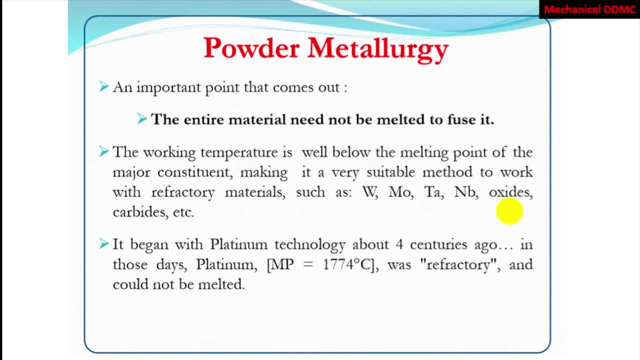 to fuse it. it means in powder metallurgy technique we are not melting the metal completely to produce some parts to convert metal shape. it means we are using it in from a multi-momentы Itu Mo. this is the very suitable pointed metal. this is the some most important things for power metallurgic. 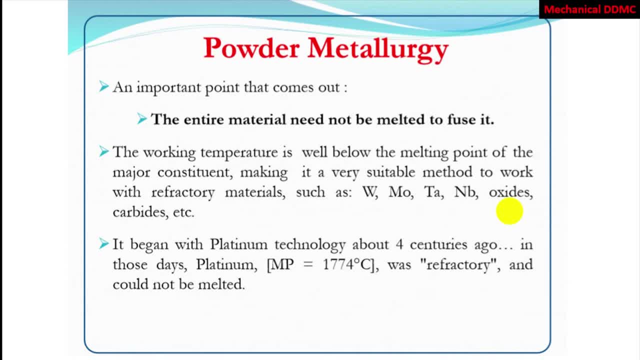 the working temperature is well below the melting point of the major concerned, making ita very suitable method to work with refractory materials such as wya, mo ta, ENB oxides and carvats. it means if we are able to shape our the metal below the melting point of heat, then i 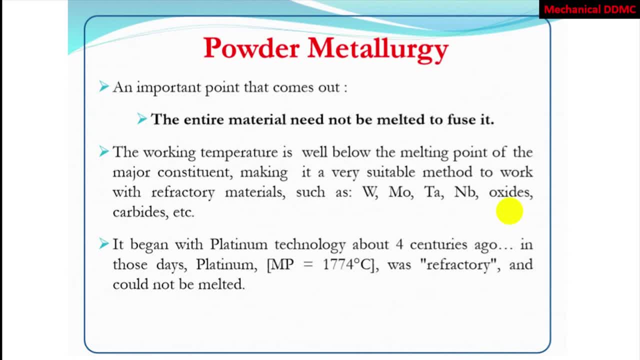 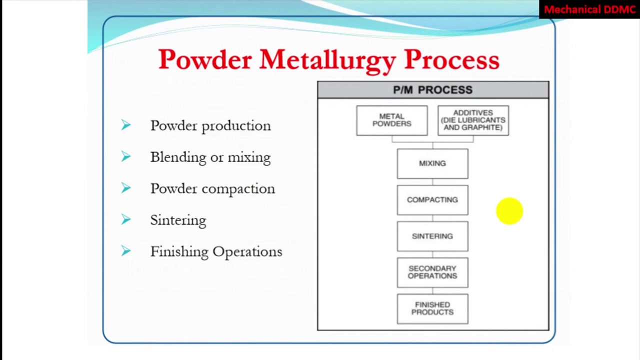 metal below the melting point of heat, then i. there are lots of advantages you can get from it. like, especially like in refractory metals materials. we can use it. okay. powder metallurgy process. before the powder metallurgy process: start from powder production, blending or mixing power, complexion centering and finish operation. okay, like in other metallurgical. 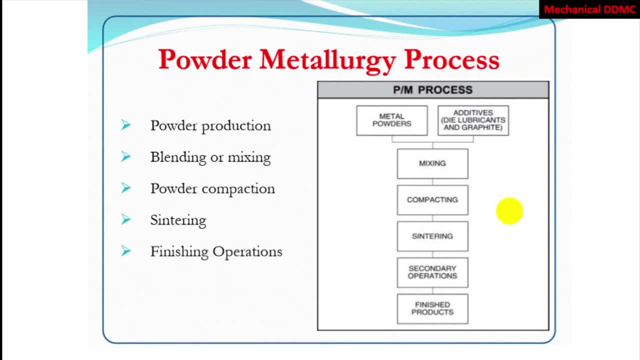 forces, powder metallurgy forces- also contains some steps. first, one is powder production. okay, powders production is nothing. it is nothing but a formation of powders from the ore, component or ore metal like uh, if we are to use or if we are to take some of the material we are going to take, some of the material we are going to use. 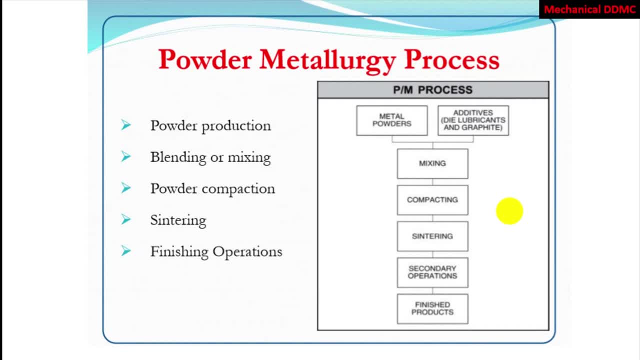 some shape of materials or components from uh iron, then the power production means the production of the iron powder. okay, and um, one thing, important thing in powder metallurgy is: uh we are using um much more than two metals, or we are using the alloy of different metals which are 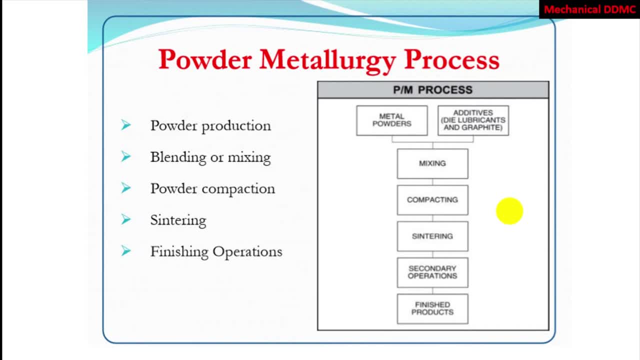 uh not capable of using in other metallurgy process. so that we are using in this process is always okay. that's why in powder production means production of the different powers from different metals that we are using for making alloy in power, material power, metallurgy process: okay. blending and mixing uh power complexion and centering. 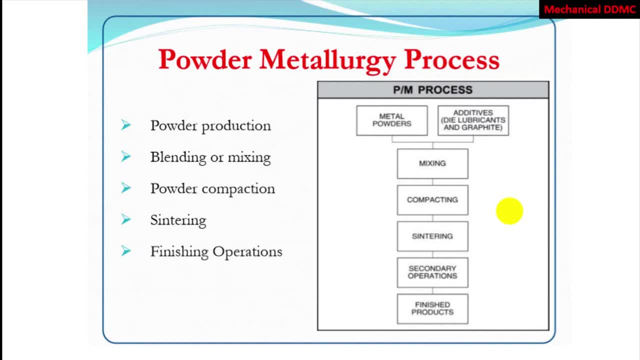 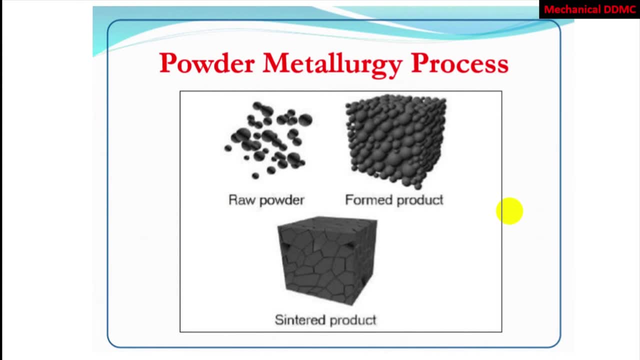 and finish operation. about that i will explain in next slides. powder metallurgy process means raw powder, that i explained. it means the powder of the raw material, raw metal. and form product means uh, we will mix them and uh, we will make some. joint action means we will form some cream shapes and then we'll 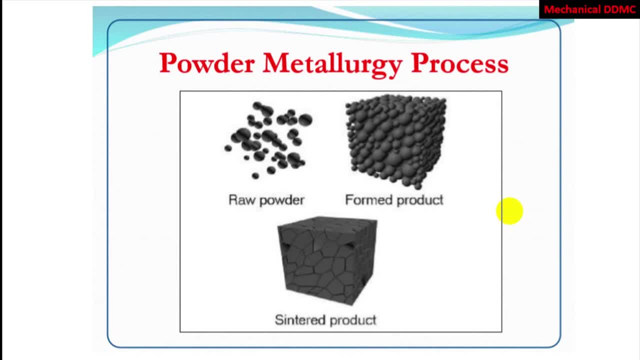 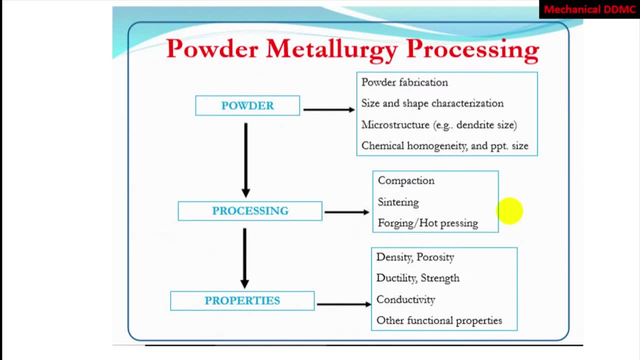 center the product and uh we'll find some strength, highly strength and density. density product: okay, here we can see powder metallurgy processing means powders, formation, powder, uh. powers also there are. some. capacity of the power means size and shape, characterization, a microstructure powder, uh. chemical homogeneity, uh. ppt size and other more uh. these are the. 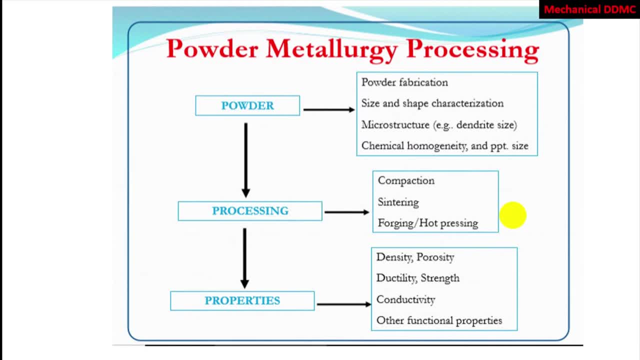 character of the power uh, which are should be studied before the procession and in possession uh the powers will become goes for compaction, centering and forging or hot compression, and after that uh we'll get some properties of our desired product. that means in terms of density, porosity, ductility, strength. 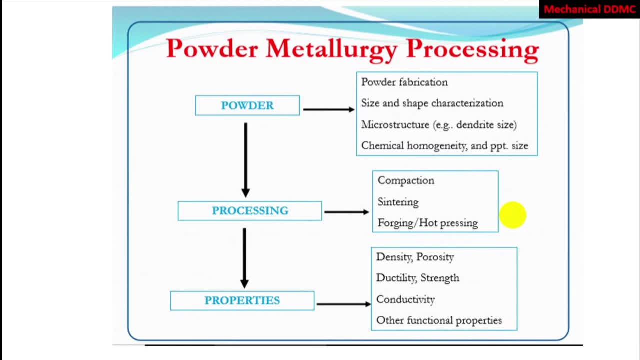 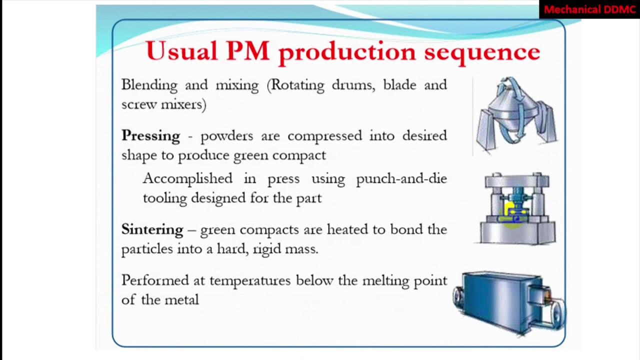 conductivity and other functional properties, that these properties are the properties of our product. okay uh, usual power metallurgy production sequence means after production of ah mean electric motor vessel. we normally make moka, and of course this is the technique. and here do a measure: sorryёт uh load from the polar in powder, so it uh. 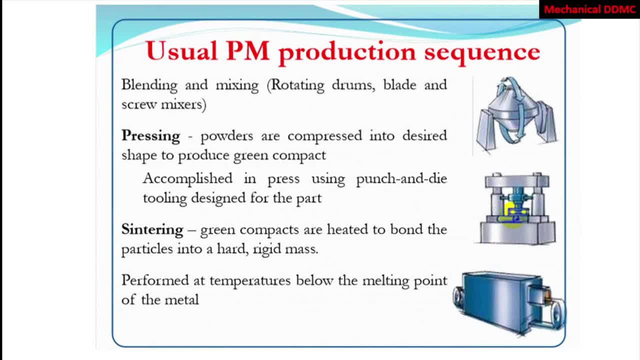 remains for hours after and we basically mix these uh components in pressed on a different way. so throughout the process we are finely co- personalized and in the way of making different uh modeling process and that means we have to really work on it uh and turn our 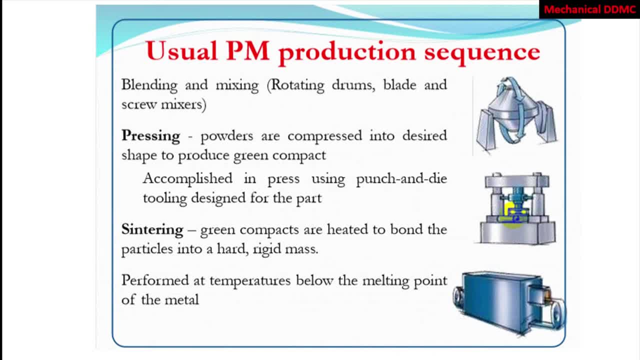 uh method of handling, the uh pleasureえ то sot reset method, but it uh forms a joint between them. they will be compact, they will pressurize to give some green shape. okay, not in color, okay, green compact. we will call green compact. and centering means 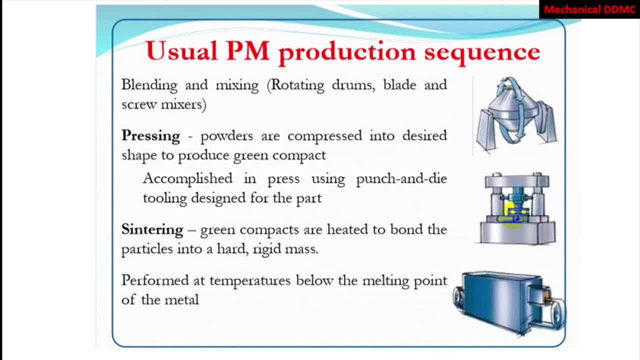 green compacts are heated to bond the particles into the hard, rigid mass. uh, it is similar to welding, okay in higher temperature. when particles of the same metals or different metals are centered or treated with heat, then they will be bonded each other and, uh, they will compact it in. 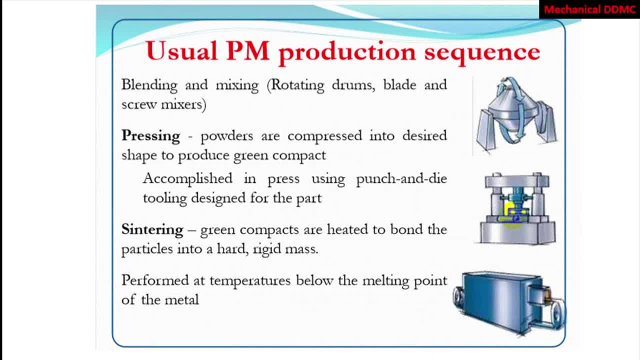 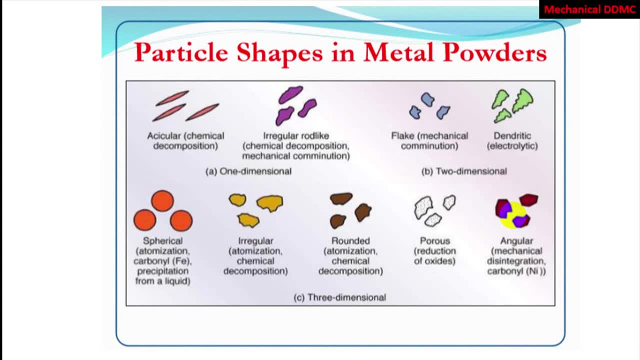 one particle or one product and uh with high strength, okay, you can get. let's see a particle sets in metal powders. uh, i already explained you that there are some characteristics of metal. powers means, uh, some angular chemical called decomposition. irregular roll like tech, like dendritic, like. 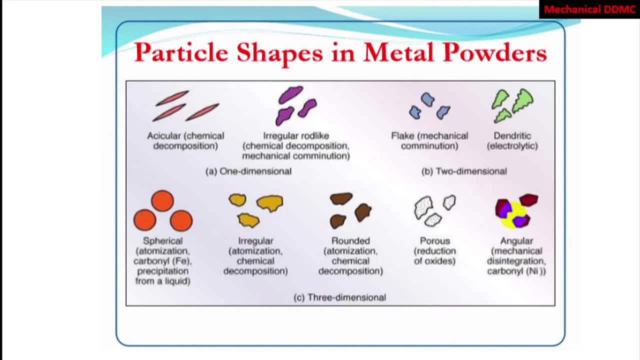 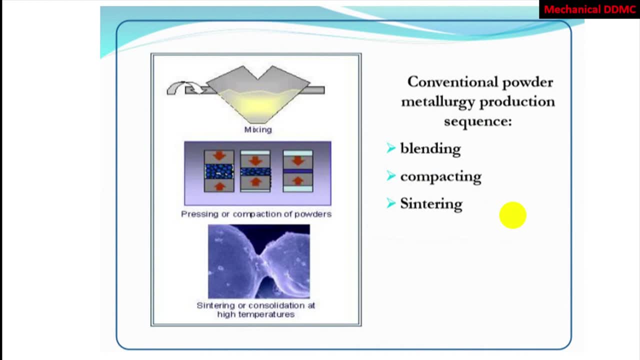 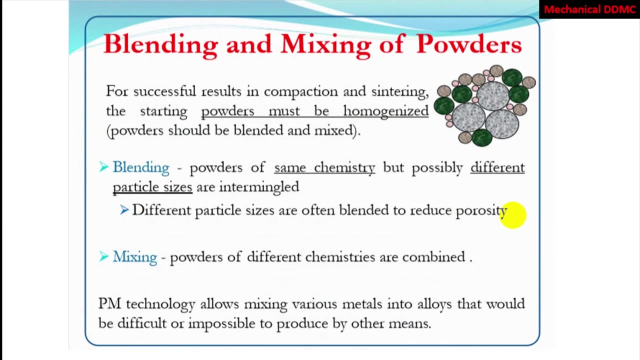 spherical, like regular, like another, more okay, uh, in conventional power metal production sequence, blending and compacting and sintering will be there. blending and mixing a powder- uh, i already told you that blending and mixing is nothing, it is just. mixing of the powders in some way means we can't just 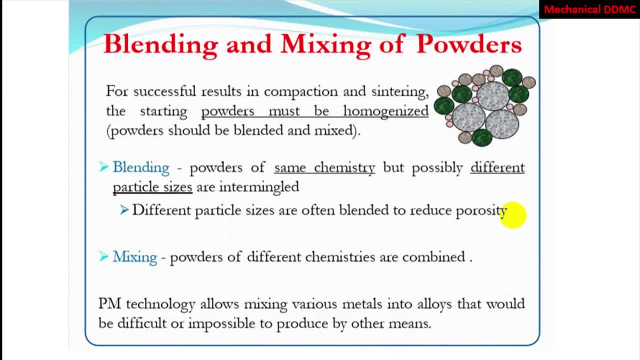 mix them. there are some criteria so that we can mix them. for successful result in compaction and centering, the starting powers must be homogenized. powders should be blended and mixed. here you can see there are different metals, um that we are going to make our way and, uh, in between them. 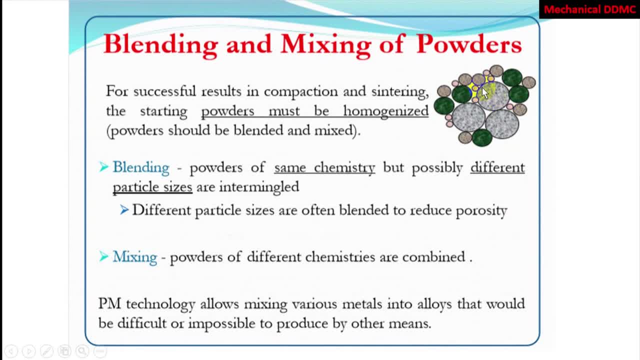 there are small particles are pleased. uh, we have to mix them in such a manner there. the size of these grains and particles, uh, should be mixed in in such a way that there should be a small gap at a very small gap there should be. our motto is to eliminate those gap with small 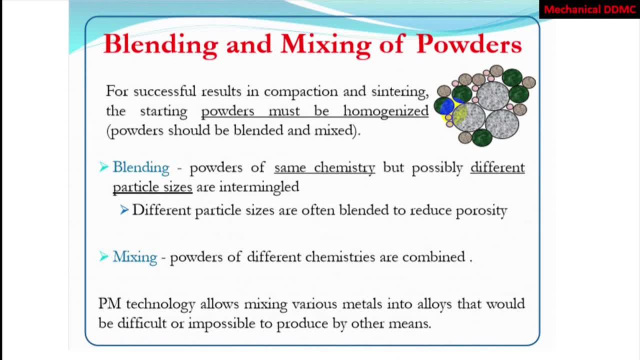 powers okay, so that we can compact them in good way. blending means powers of same chemistry but possibly different particle sizes are intermixed. means in blending we will mix the powders of same chemistry. means same material, like uh iron. we have different powders with a different size, uh shape of iron. 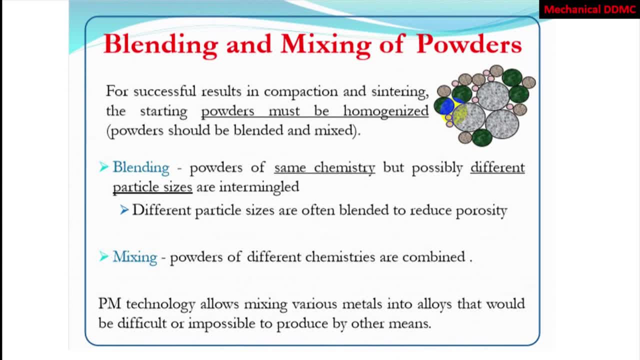 they will be mixed each other means having same chemistry but a different size, so that, like you can see, this and this could be iron. they are mixed each other so that the space between the this and this could be filled by iron. only means same chemistry, but possibly different particles. 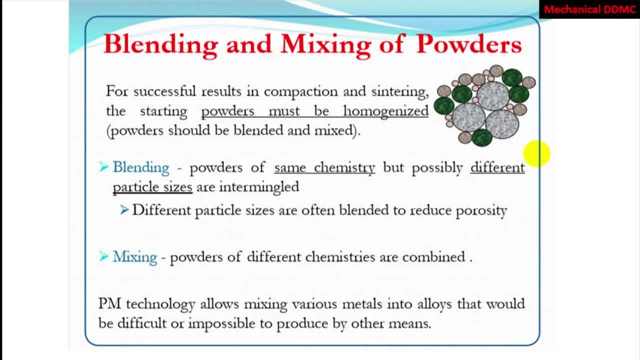 are intermixed so that there will be a greater possibility of intermixed between them. different particle size are often blended to reduce porosity. okay, and i already explained that it reduces the porosity. this cap reducing means porosity reduces and mixing powders of different chemistries are combined. means in mixing powders of different metals can be. 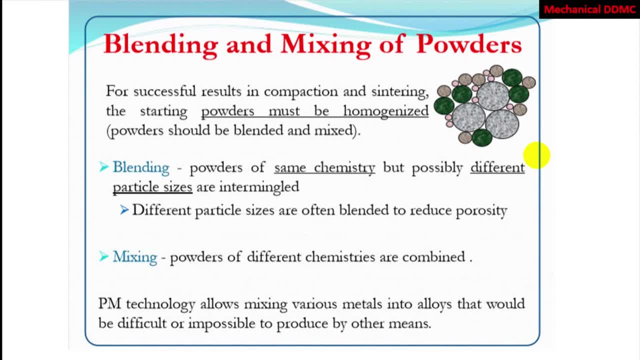 metals and non-metals also can be combined. this is called mixing powder metallurgy techniques. always various metals into always that would be difficult or impossible to produce by other means means, uh, in other or in our general sequence we may not be mix those metals into always. 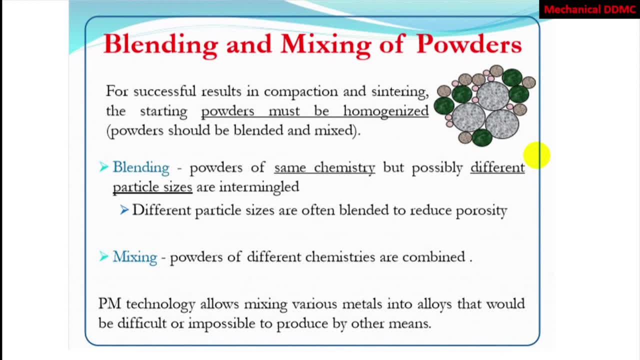 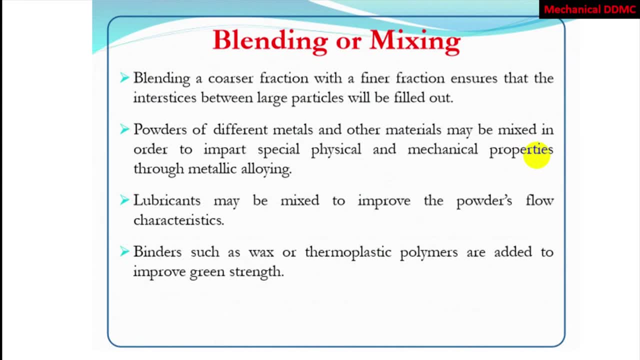 but powder metallurgy techniques give us to allow mixing various metals into otherwise. okay, i'm blending and mixing. blending is a coarser fraction with a finer fraction ensures that the interstatics between large particles will be filled out. i already explained that there can be gap between two large particles, so that if we allow some small sizes, 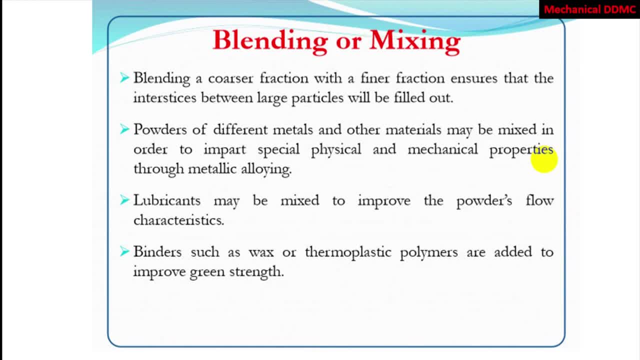 small size powder into between them, then there will be a greater mixing. okay, that's right, it is called blending and powers of different metals and other metals may be mixed in order to impact special physical and mechanical properties through metallic alloy. okay, uh is for mixing, means if you mix different metals, powders, metallic powders. 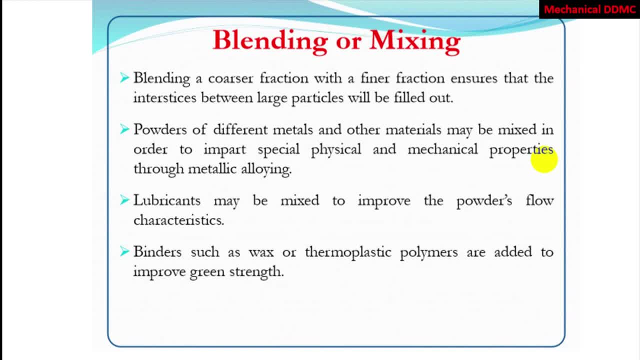 then, uh, its mechanical and physical properties will be high. not only mechanical, but also physical properties will be high, high than previous one that is called alloy. lubricants may be mixed to improve the powerless flow characteristics. uh, in this stage, we can also use some lubricants so that they will improve the 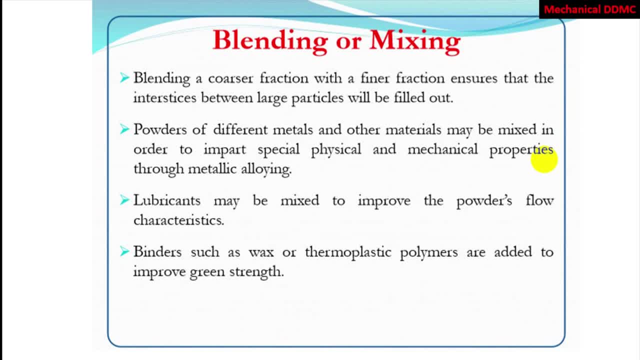 powerless flow back characteristics and binders such as wax or thermoplastic polymers are added to improve being strength. green strength means uh green, strength means uh green. after compaction they are not fully mixed but they have some uh shape already, which is none of the green. 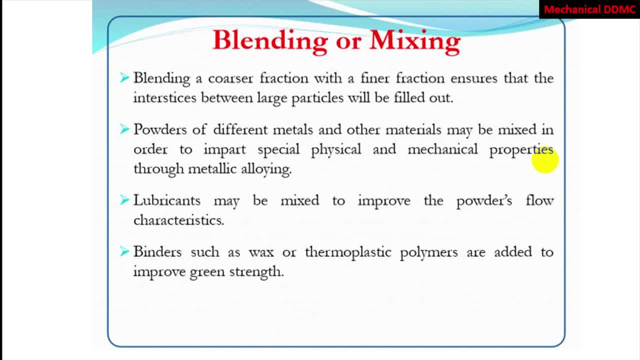 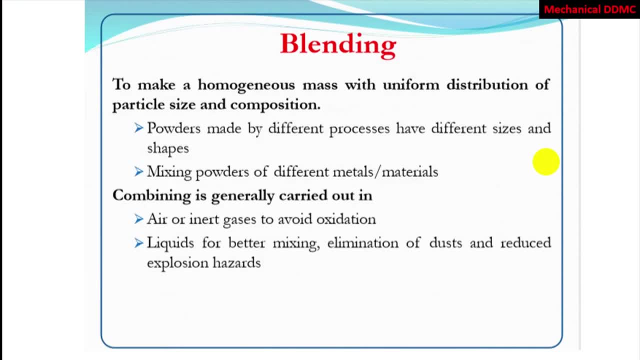 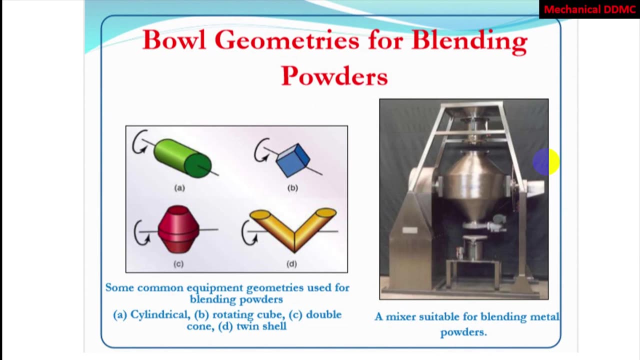 product or green strength. okay, the strength of this product is known as the green instant after the compaction. only this is already explained to you. and world symmetry for blending powers means for blending. blending means a mixing of uh, a mixing of same materials, for us, okay, having same chemistry. here you can see, this is. 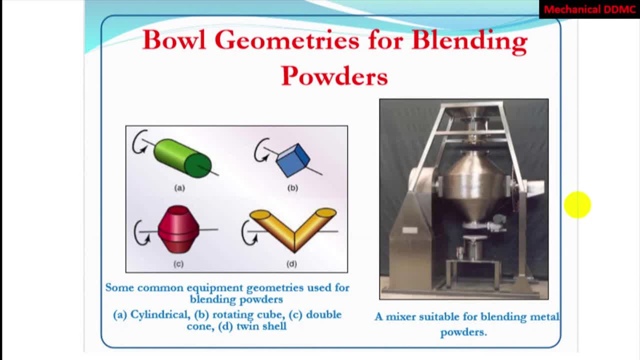 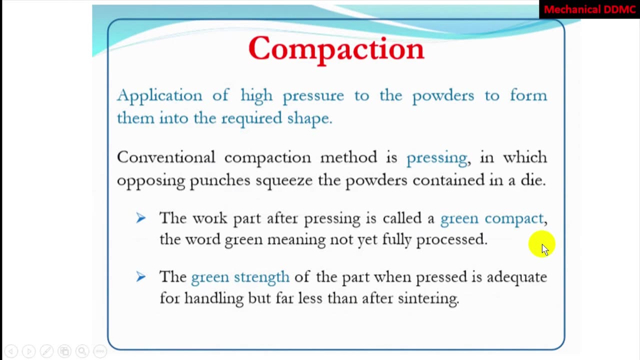 balls. images for blending powers means this is a ball with cylindrical shape. uh, it can be rotated so that they can be mixed. during this rotation you can see, and compacts application of high pressure to the powers to pump them into the required set. this is the very important station parameter, like techniques. 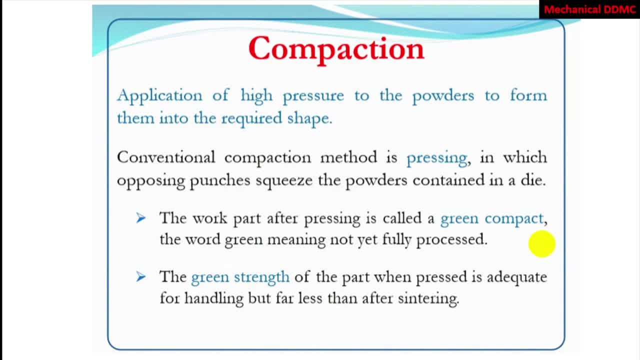 means, after the formation of power, they will be compacted through the fire pressure to the powers to form them into the required shape. and this, uh, this gives the shape of the our product required. okay, conventional compaction method is placing in which the opposite punches squeeze the powers. 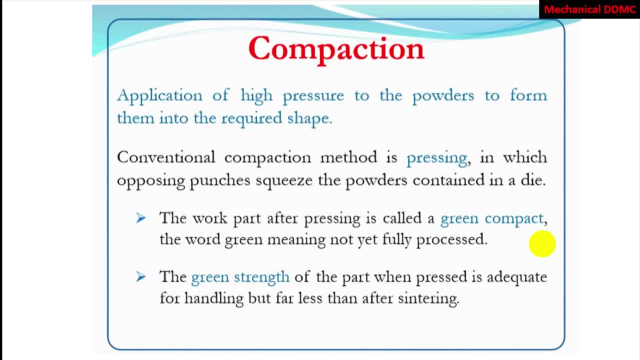 contained in the dye means it is similar to pressing, where we'll put some powder, mix a powder. after mixing we will pour into the dye or into the pressure pressing machine and then we'll press and it will give some shape, like in die casting. okay, the work part after pressing is called green compact. the word green means not yet fully. 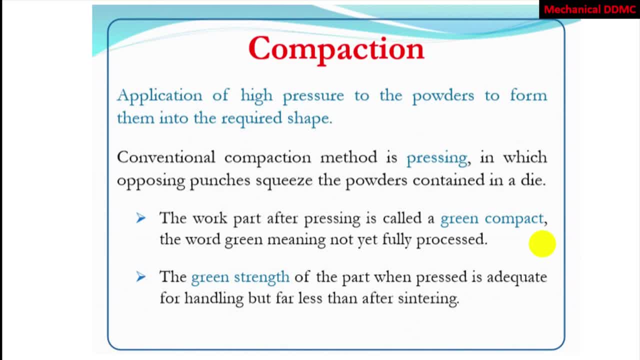 press. it means they are not totally mixed or they have don't. don't have a greater strength, but size is already we got. okay, after a compaction we can get the size, the powder required, but that product is not fully strengthful. this is called- uh, so it is called- a green compact, the green strength of 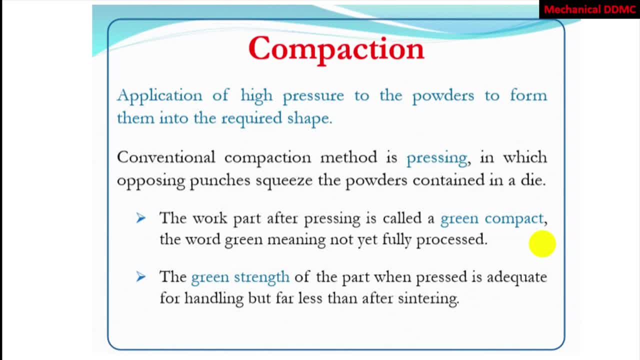 the part when paste is adequate for handling, but far less than after century means, uh, they only mix in a solid form, they are not totally mixed. but they are not totally mixed, but they are not totally mixed. also is that: or they have a strength for handling only to transfer from one place. 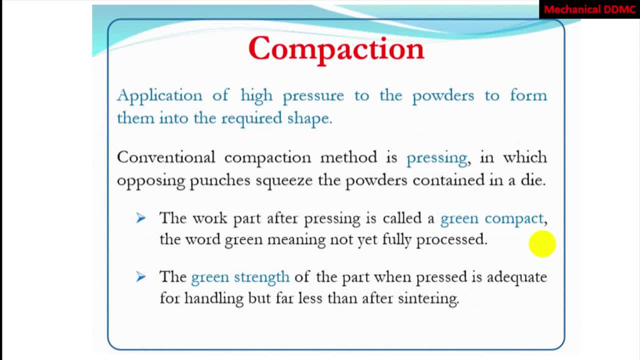 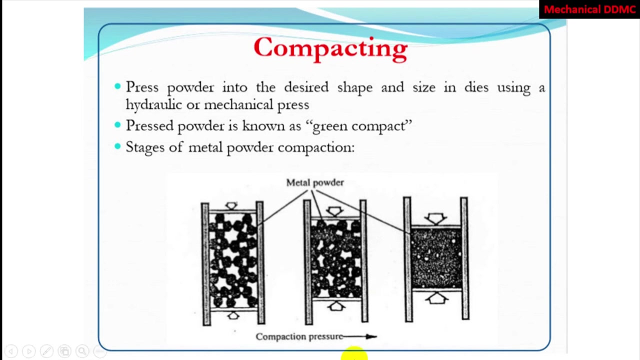 to another place. they will be capable, but not for our use. not for is, after centering, okay, to change the strength of, to increase the strength of the product. after compaction, we use sintering process. let's see here you can see compacting and we can give pressure from top or bottom or from both sides. there the particles will 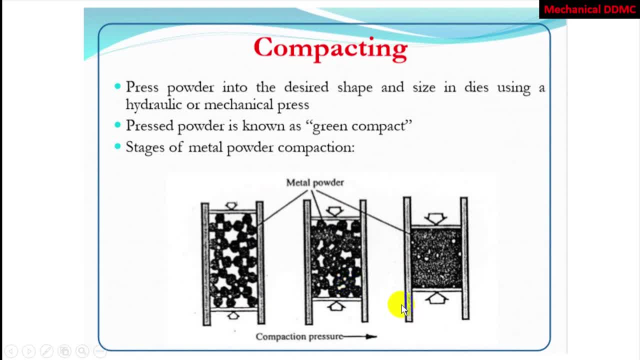 become closure and after high pressure they will be like one shape or one product. we can change the shape die so that the product after the comparison will give the final size of the required product. okay, the place powder is known as the compact, green compact. this is metal. 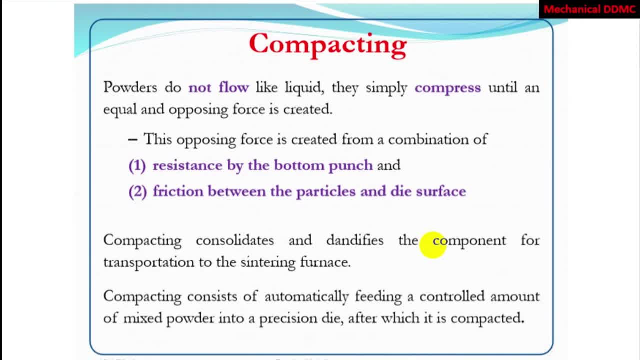 power compaction. um, here is. this is similar to our, the casting in die casting also. powders do not flow like liquid, they simply company is until an equal and opposite force is created means or we don't need a, we don't need to melt a metal, just powders do not flow like liquid. 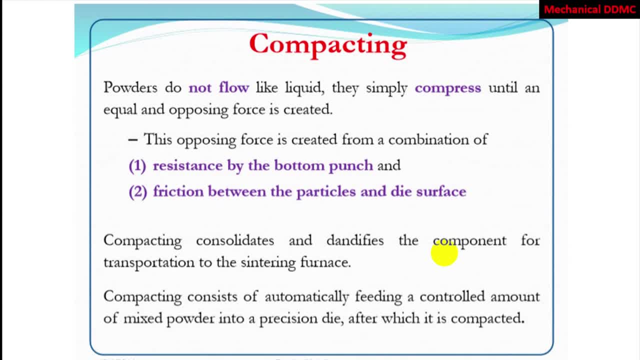 just simply compress until an equal and opposite force is created. This opposing force created for a combination of resistance by the bottom points and friction between the particles and die surface Means, due to the friction and due to the resistance from the bottom points, that is force. 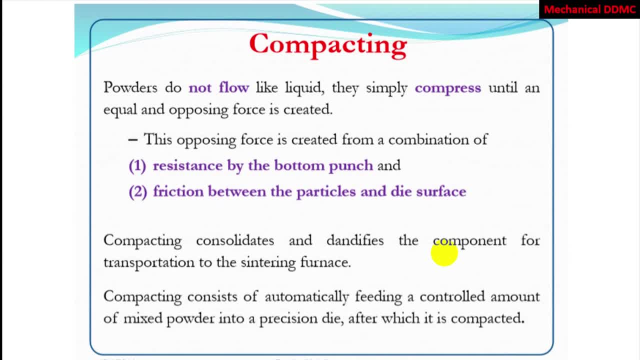 have applied, they will be compressed and they will form the shape that we required at last. The compacting consoler identifies the components for transportation and sintering furnace Means. after compacting it will give the final shape, so that, so that, sorry, after compaction it will give some shape, so that 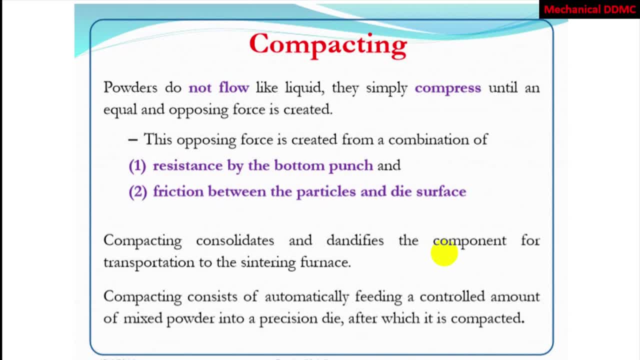 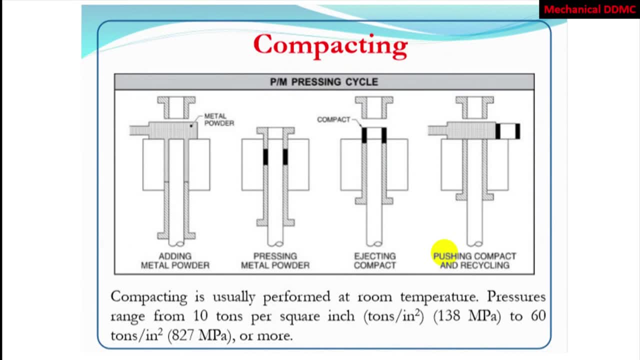 we can transfer it for transportation and sintering furnace. okay, Here you can see the process of compaction. here we can put metal powder through. here this is metal powder for our final shape and after compaction we can remove it from here. okay, we can remove it from here and this is the. 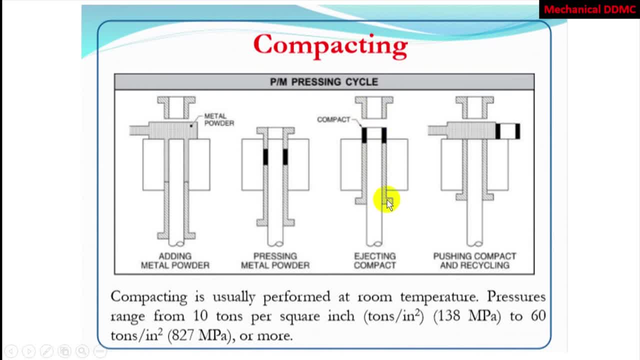 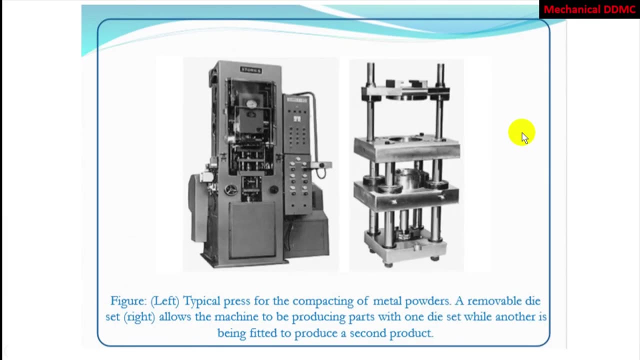 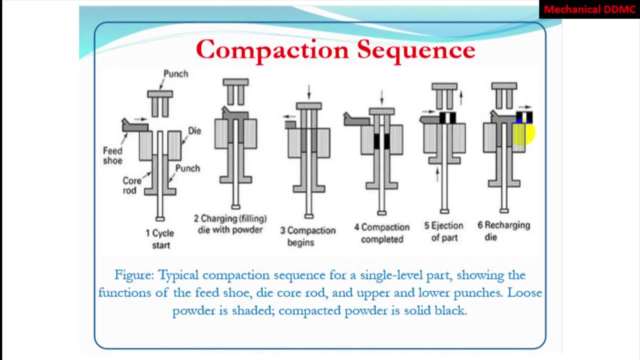 upper punch, and this punch can be stationary, and then, after applying application operation, these powders will be compacted and after that, after compaction, we can get this final size. okay, This is hydraulic compaction machines- compaction sequence. yes, you can see this. also. this is similar to this one, uh, where we are. 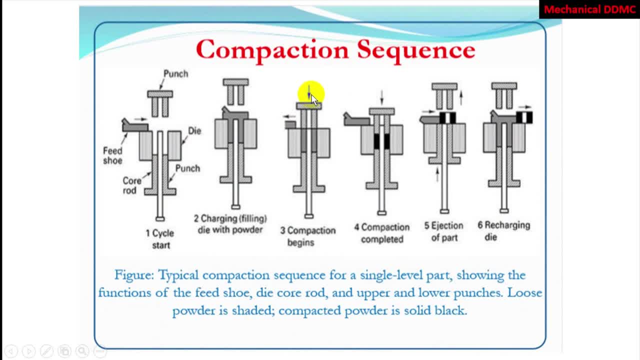 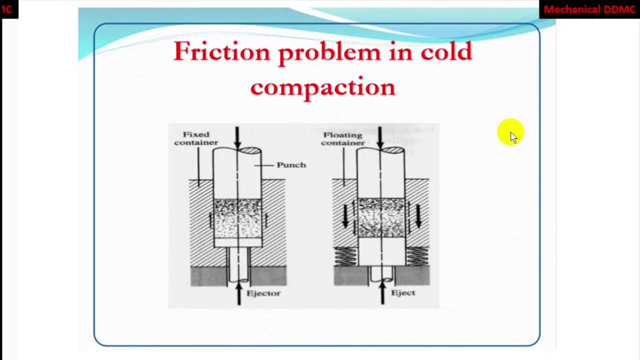 placing from upper. okay, we are placing from upper. uh, this bottom punch is stationary and after the compaction completes the compacts. after compaction, the green compact will be throughout from this one and uh, take it to sintering, sintering, heat treatment to burn the. 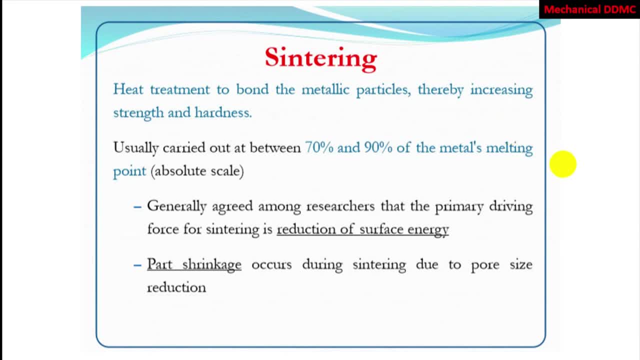 metallic particles, thereby increasing strength and hardness, means after compaction, uh, we can get the final product that we are required, but that doesn't have the high strength that we require, that doesn't have the high quality that we are requiring, uh, in this way, the heat treatment to the 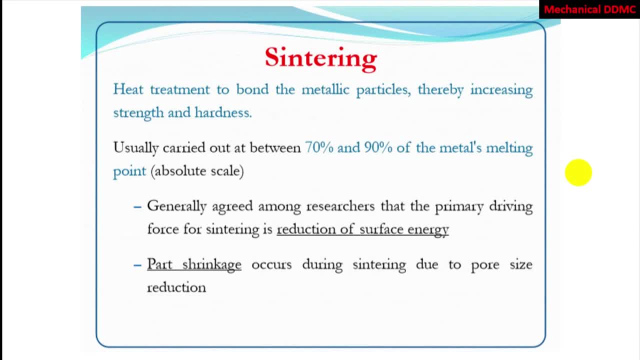 bone to burn the metallic particles, thereby increasing the strength and hardness, means uh. i can give the example of the welding, where in welding, also uh, two metal particles will be bonded together in high temperature. in similar way, here also in sintering, uh, heat treatment will be given. 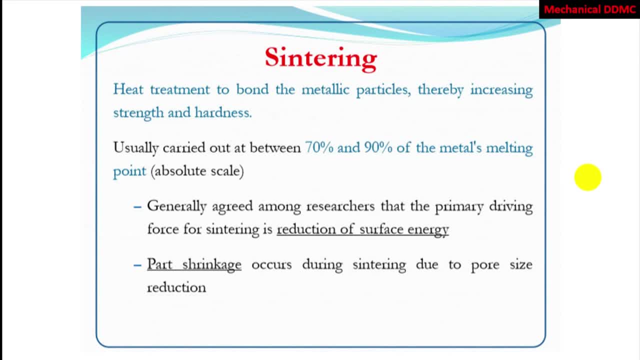 to that shape after compaction. so it makes the bone between these particles, means these powder particles, thereby increasing the strength and hardness. uh, since, uh, they are not totally powder, also because they are already compacted. it means, uh, it creates the bone between metallic particles, thereby increasing the strength and hardness, usually carried out between seven and eight. 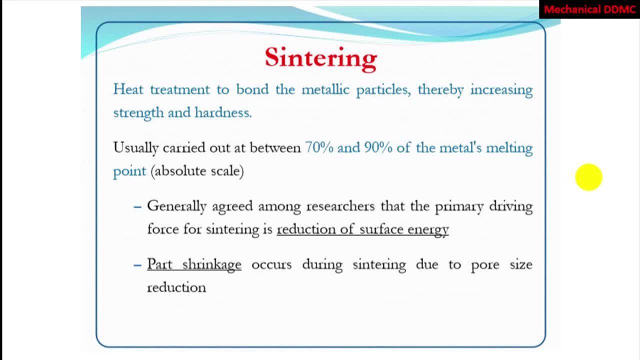 70 and 90 percent of metal melting point means we are not melting totally. in sintering we are providing 70 to 90 percent of the melting point of that metals or similar metals generally agreed among researchers. there, the primary driving force for sintering is reduction of surface energy. 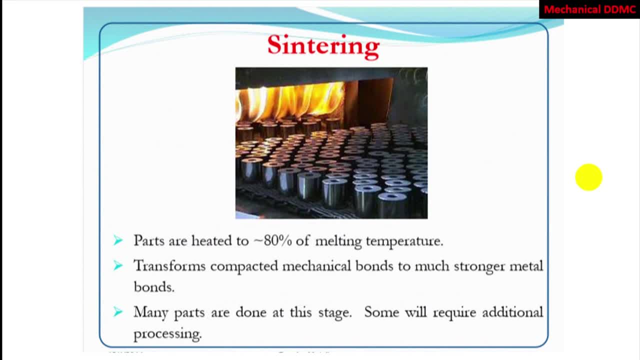 okay. sintering parts are heated to 80. nearly 80 percent of the melting temperature transform compacted mechanical bones to much stronger metal parts means uh, as in like in curling, the metal particles will be bonded each other in small manner. means in mechanically and. 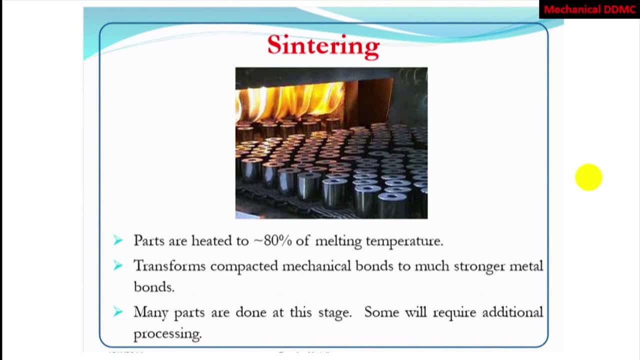 metallurgically they will be bonded each other and in a shape that is required for final size. they will be bonded means they have high density and high strength and high quality and so that it will be stronger. many parts are done and in the 60s some will be required as a stop for session. 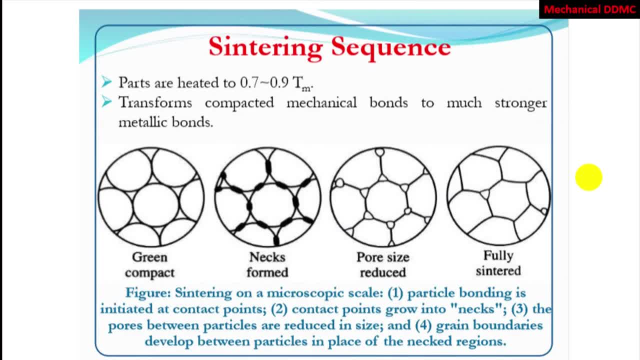 centering sequence means parts are heated to 0.7 to 0.9 means now up to 90 percent, or temperature of the melting point. transform compacted mechanical bone to much stronger metallic point. okay, or they will change the shape of greens, shape of grains of the metals. 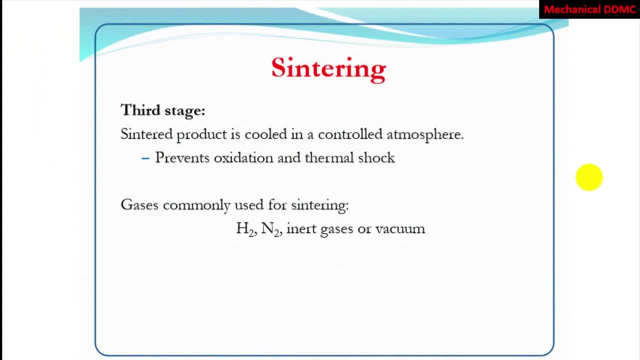 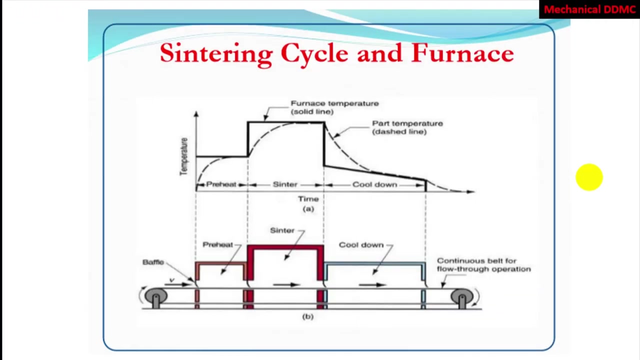 in third stage, center product is cooled. in a controlled atmosphere means after heating or after centering it will goes to cooling, and cooling control atmosphere prevents octation and thermal shock. gases commonly used for sintering are s2n2 inert gases or vacuum. you can see this sequence of 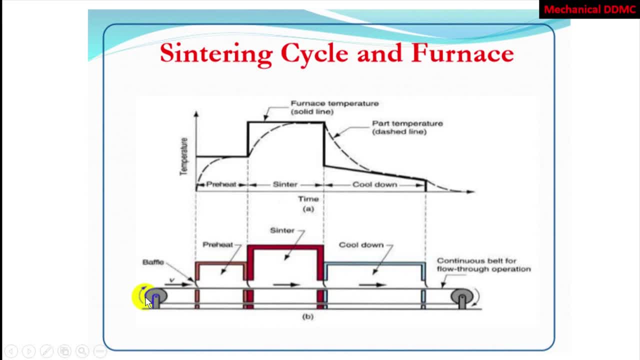 sintering. here we can see this is a rotating and here the particles after the compaction will be coached and it will be preheated. and you can see, after paint preheating it is go to sintering furnace and it will be heated. you can see this. 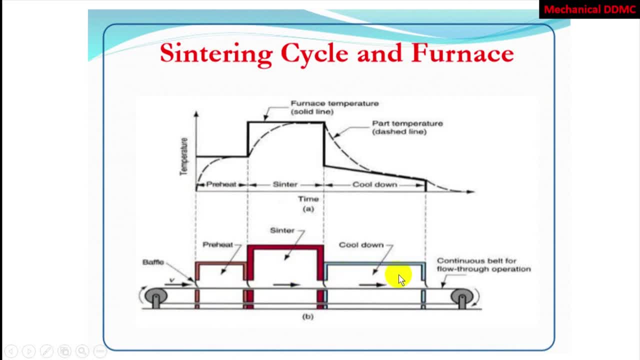 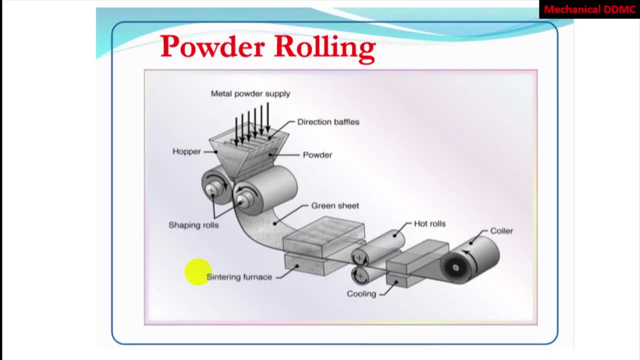 this is sintered and it will goes for cool on and again the parts and the parts will be repeated. if you can see, the powder rolling process also means some powder to some safe. some have said we can polish. this is similar to this. our order, metal energy. this is total power, manly technique, but in a different. 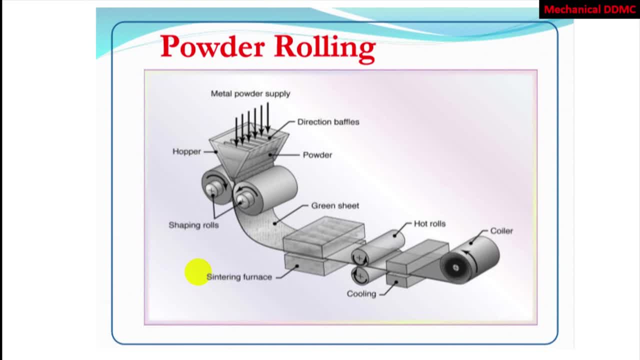 way we are using this instead of 4 die supercomputing, wait using roller. okay, stepping rules here. we were going going to sip top powers into some cast simplement it. this is another green sheet. okay, crazy, and it comes with sintering finance here, or it is heated. 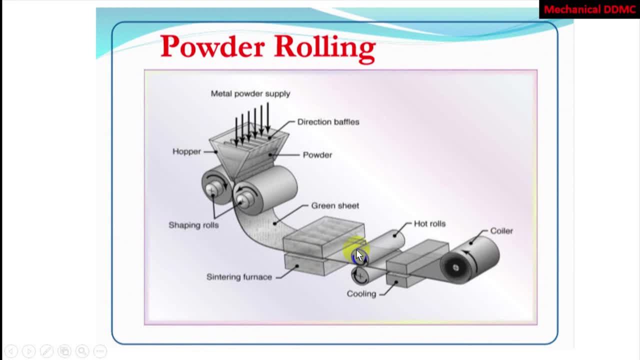 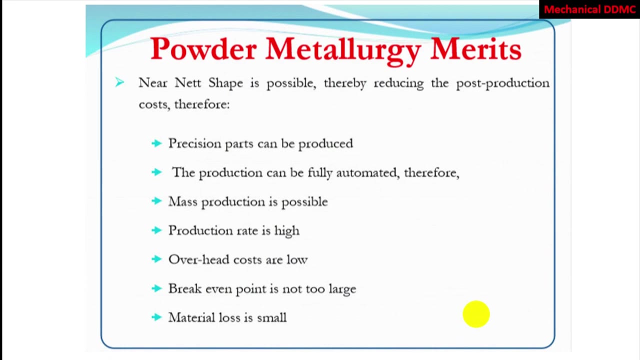 and bones will be ferment form and goes to hot world for the required shape and goes to cooling and it will form uh required parts. okay, uh, let's discuss about the power metal mills. uh, in first, only i told you that the quality is most important. it means, in power metal techniques, the parts are. 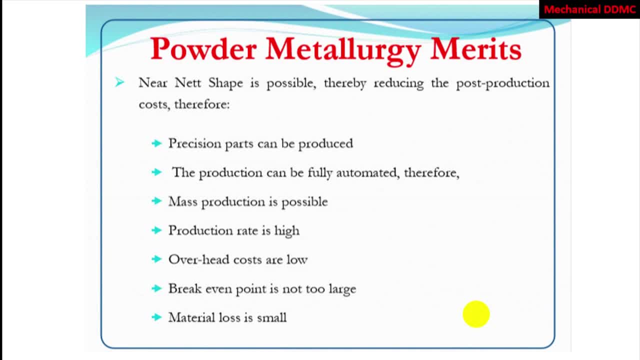 accurate, with high quality and high strength, with good mechanical properties that are required. that's why only power metalers techniques is famous for these days, like a bmw cars and in other aerospace and engineering terms also. uh, they're polishing aerospace engine. uh, they're polishing these types of parts. 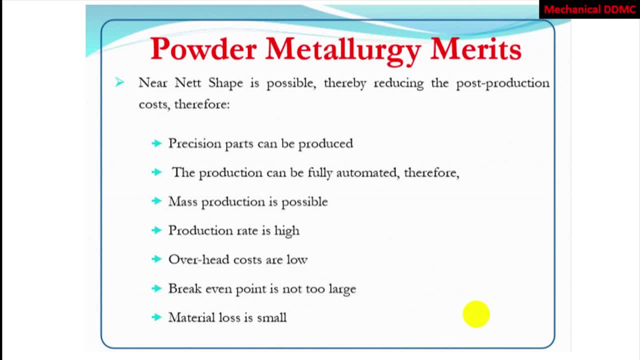 uh, which requires high quality. they're polishing through the power metal technical because after power metal techniques the machining required will be less, very less than other machine parts. other parts is okay, precision can be for use. the production can be fully automated. the mass production is possible. okay, production rate is high. overheat overhead cost are low because 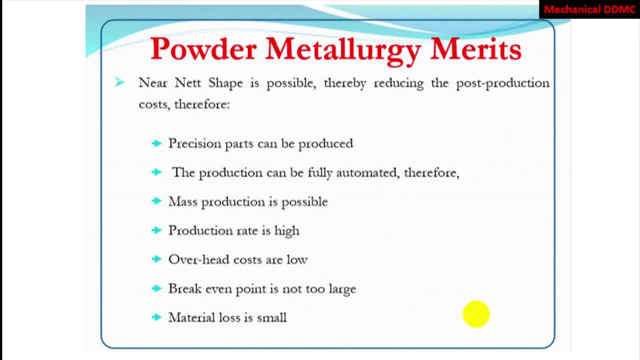 uh, the machining requires a load. that's why the given point is not too large. metal loss is small because we are polishing the required shape at last through this force. okay, our master, important thing is the quality and strength of the power that we are getting from the mixing of the different. 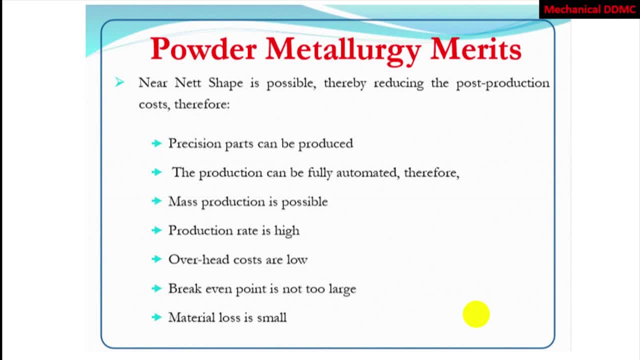 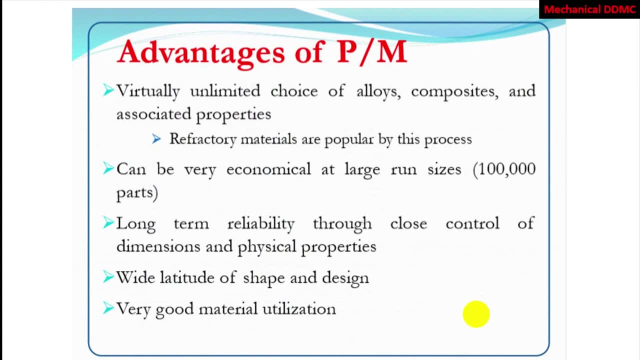 metals, uh, which may not be uh generally possible from conventional metallurgical forces. uh. virtually unlimited choice for alloys, composites and associated properties. means are different alloys composition, associated properties we can use refractory materials are popular by this. forces means: refractory materials cannot be heated to. 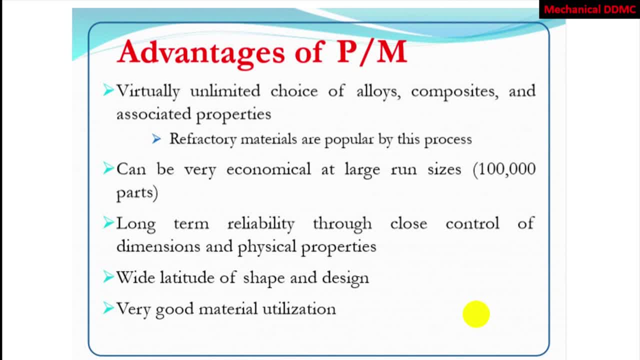 get melting point. that's why all we can use these parameter techniques can be very economically at large run, size, long-term reliability through close control of the dimensions and physical properties, while laying a latitude of shape and design means. uh, this depends upon our compaction size of machine provided. so if we, if we can increase the complexion, such a 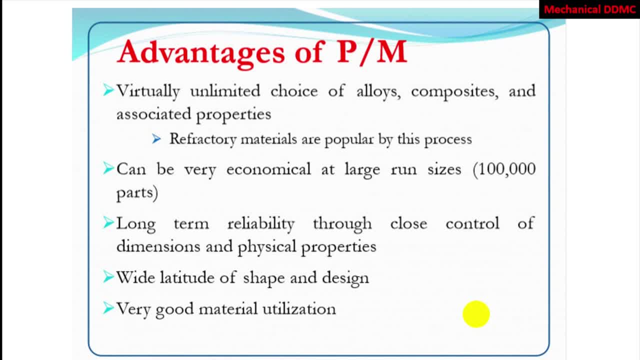 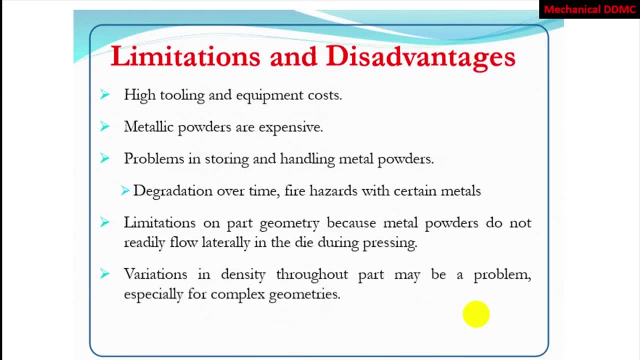 machine. then, um, directly we can make the parts bigger than bigger. very good, metallized metal utilization limitations and disadvantage high tooling and equipment costs. are there? okay, this concept, that's one. metallic powers are expensive because it takes some time and some costs to form the metallic powders. also for problems in storing and handling metal powers. okay, a degradation. 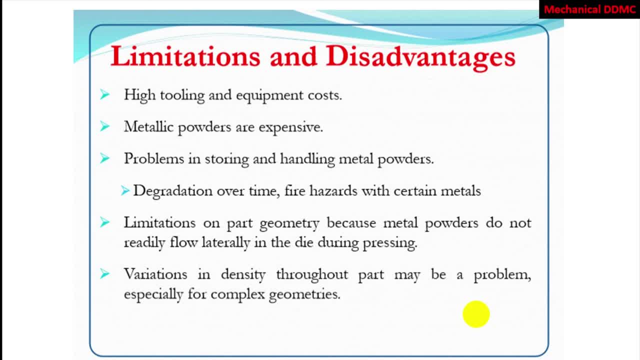 of a time fire hazards with certain metals limitations in the party. but it because metal powders do not really flow literally in the die during patient variation density throughout the part may be a problem for complex symmetries. it means in some cases there may be some difficulties too. 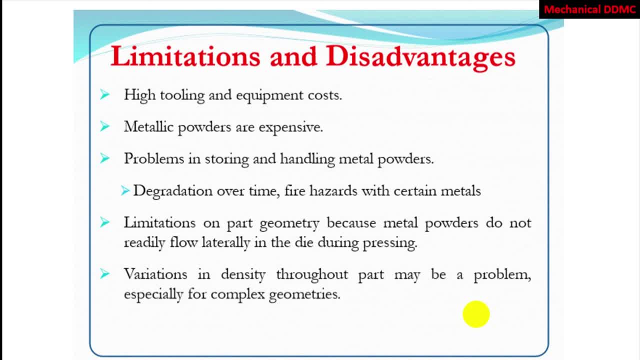 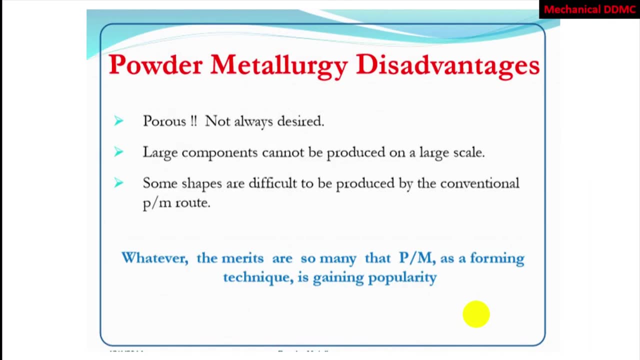 like a degradation of over time, fire hazards or limitation for fire symmetries are some example. and metallic powders are expensive means. to form the powders is costly, which may not be necessary for a general purpose, also for us not always desired means. I already explained that during mixing or 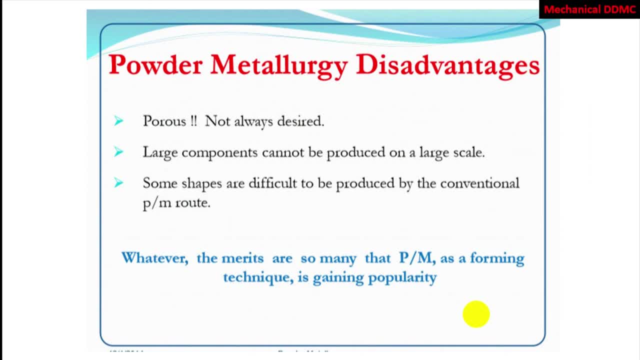 during blending. our purpose is to reduce the porous by mixing the size of different particles each other, but which is not 100%. large components cannot be produced on a large scale means we have to increase the compaction size machine, which may not be possible in all those cases. some shapes are difficult to be. 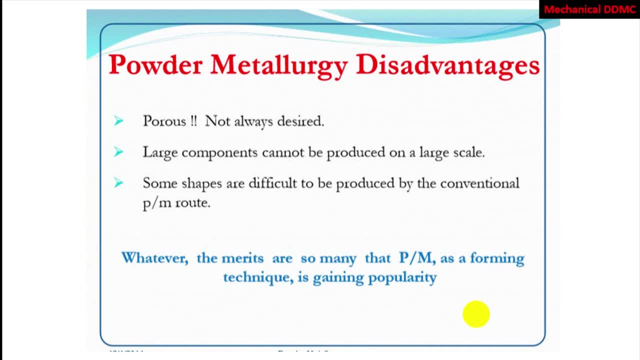 polished by the conventional powder method. okay, whatever the merits are so many that powder metallurgy is a forming technique is gaining popularity. means are to do this mostly in the various quality and sequence of operation and this strength that we are getting from. final it is going to be more popular and muster top or